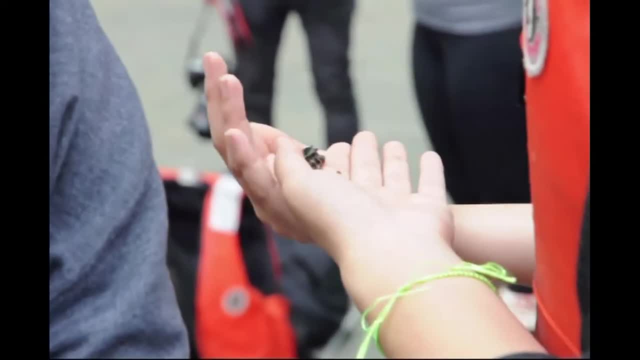 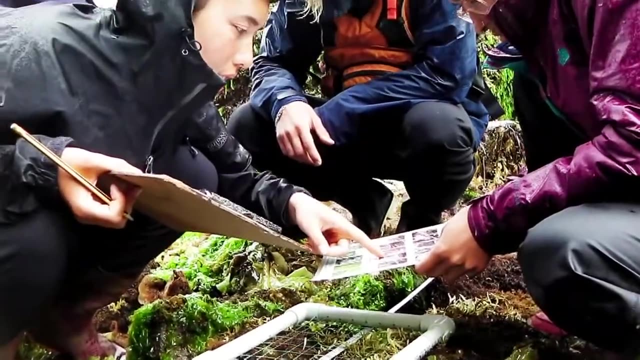 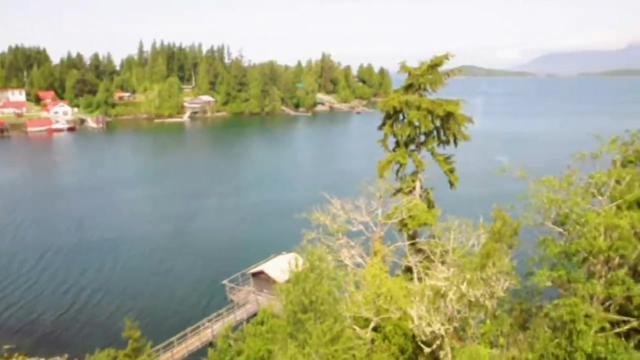 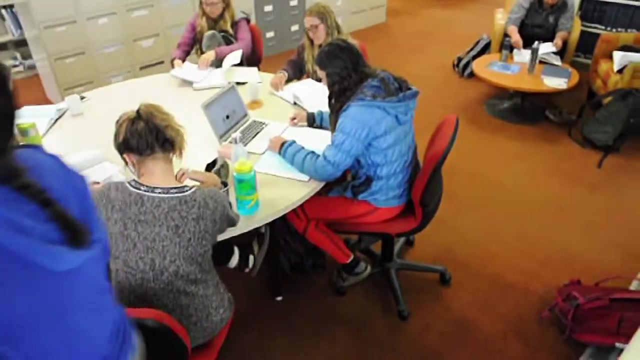 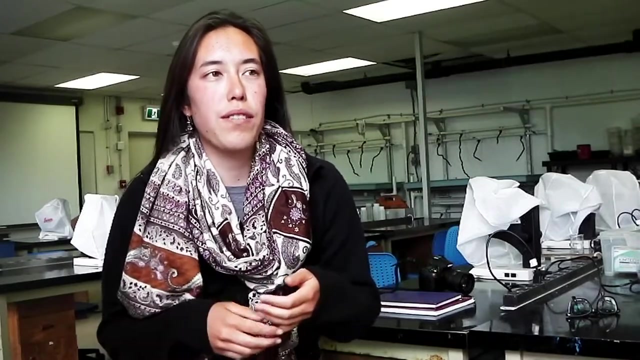 and collecting our own samples. We don't spend a ton of time in lecture, but we get out there into this really unique environment and try to learn from actually doing it, from seeing these things ourselves. This course has really allowed me to understand the tools that I use in oceanography and really. 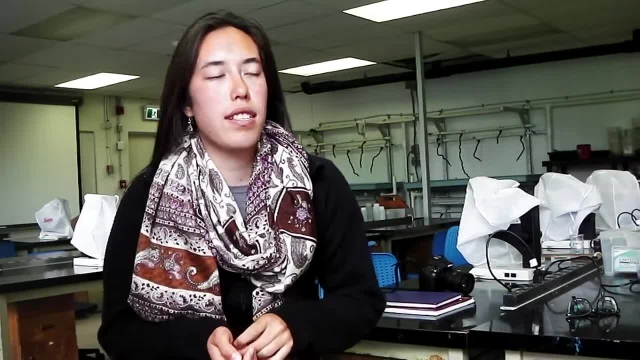 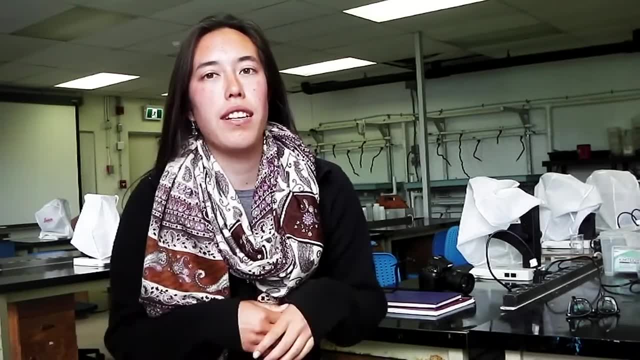 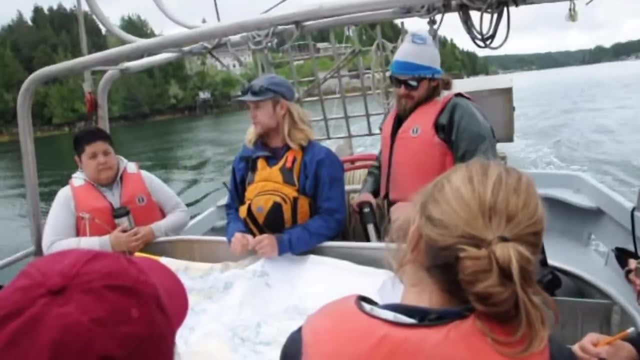 fall in love with the science behind studying oceans. This course allows us to do an independent research project, and for mine, I'm doing it on the abundance of microplastics within the oceans surrounding the UMFC, And it's been really amazing to work with other students and staff around the area and 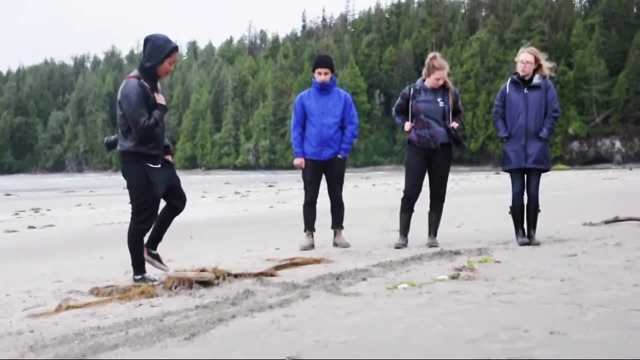 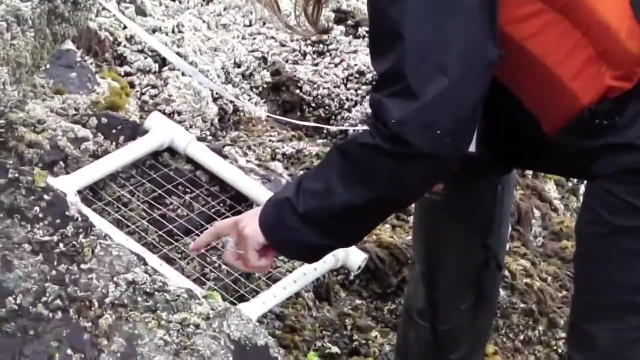 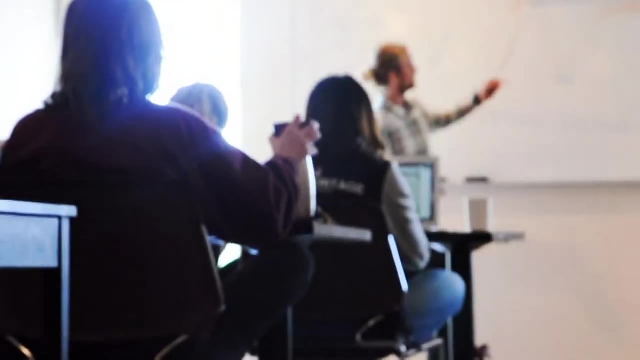 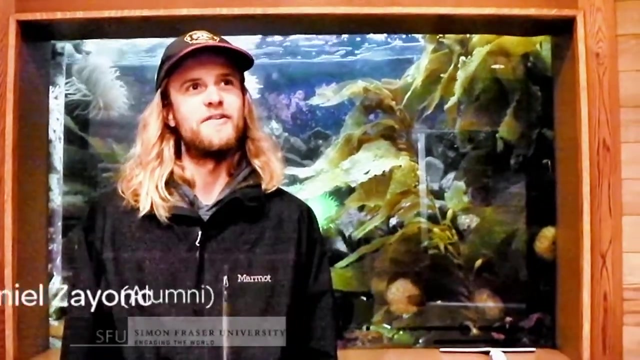 just see how knowledgeable everyone is And it's just kind of made me really love oceanography in general and want to look at future careers or kind of future research projects on microplastics. I really enjoyed TAing biological oceanography. I felt like I was super involved with making sure that the projects actually ran. 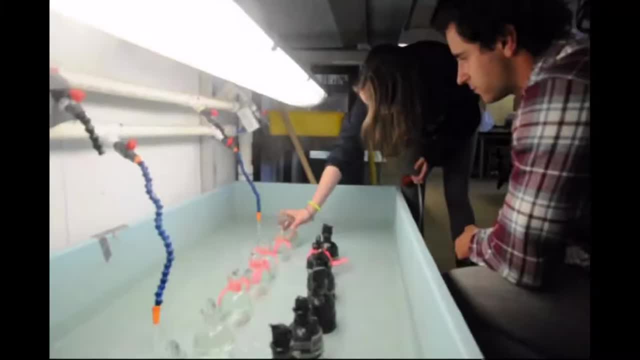 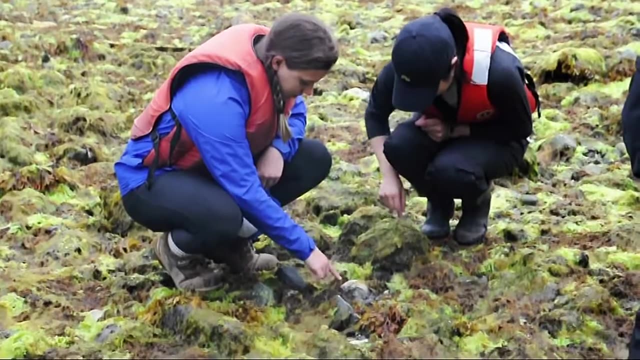 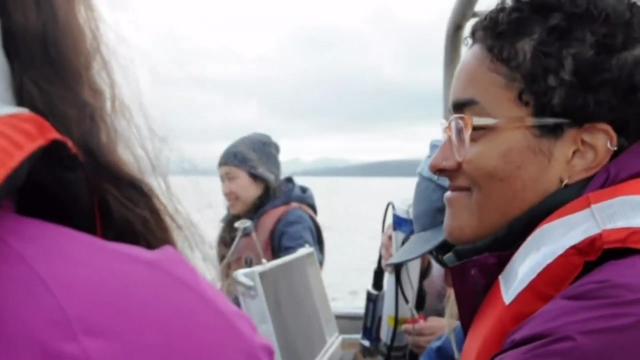 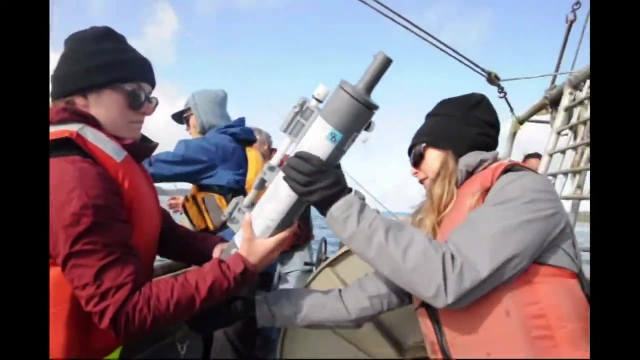 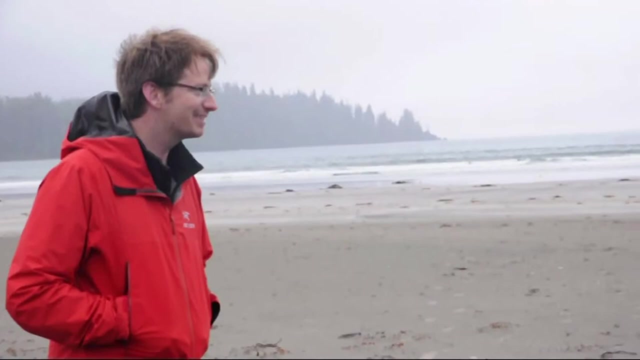 I was on the boat almost every day as a boat driver and getting out there in the field with the students was something that was pretty special And it makes me feel like I was part of the ocean and part of this of this community, And I was so happy to be part of this and part of this community because I fully enjoyed. 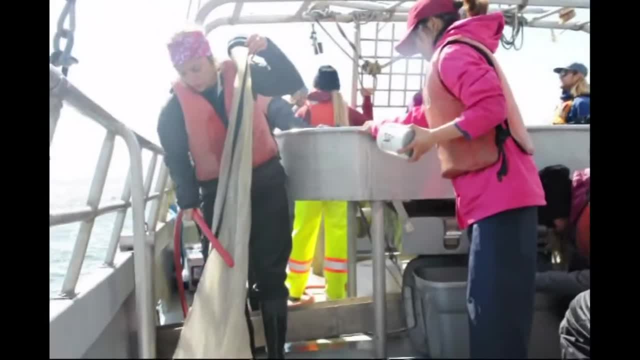 it and I think it's just been amazing and fun. This is the end of our course. If you have any questions you would like to ask, please feel free to email me that information at seonet, at seonet. Thank you for tuning in and I'll see you next time on thelets from the LA Sea. 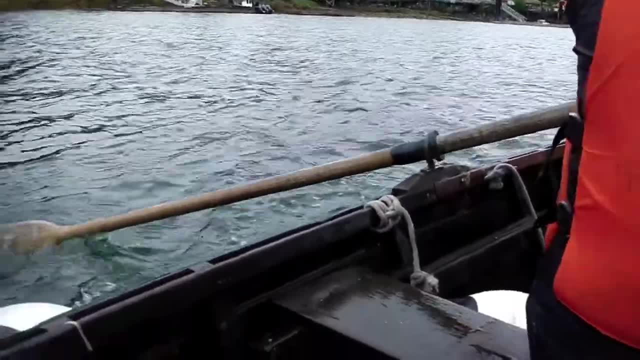 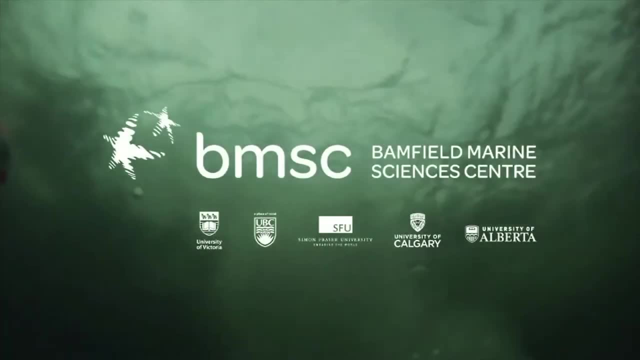 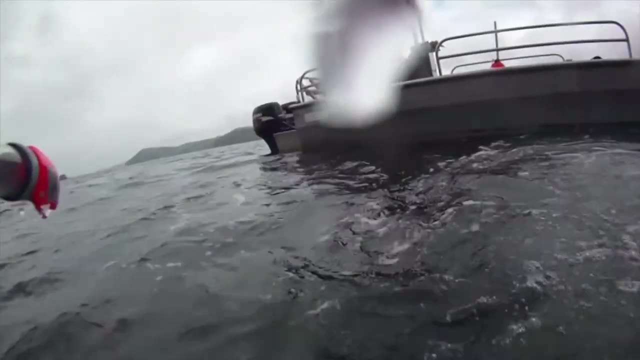 Good night. Good night everybody. See you Have a lovely day. Thanks for watching.